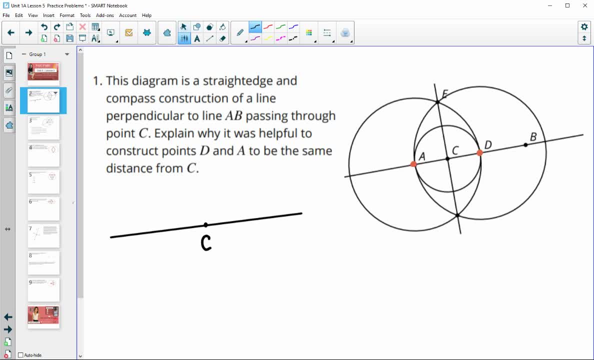 centered at C, so that we could find those points- A and D- that are the same distance away from C. So why is that helpful? And that's helpful because then- and let me just type this out as I'm saying it, Okay- Because then we would know that C is the mid-point, since it's equidistant from A and D. 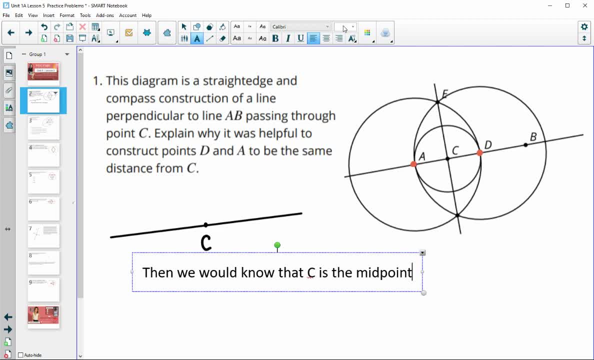 So C is the mid- sorry- A and D. So C is the mid-point of segment AB. So then we can construct the perpendicular bisector that we've done in previous lessons, which would guarantee that the line created is perpendicular to the original line. so to line CB perpendicular. 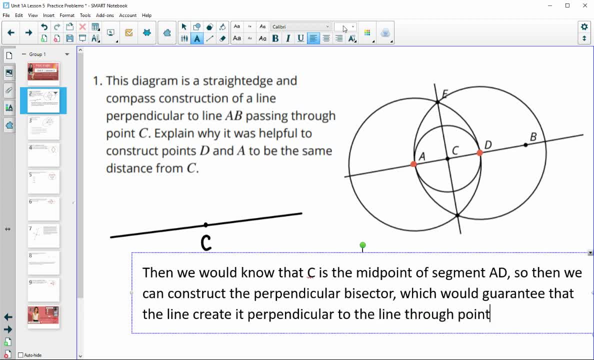 to the line through point C. The perpendicular bisector is perpendicular through the midpoint. So we just found two points to make sure that they are equidistant from C, so that C is forced to be the midpoint. Then we did the perpendicular bisector construction. 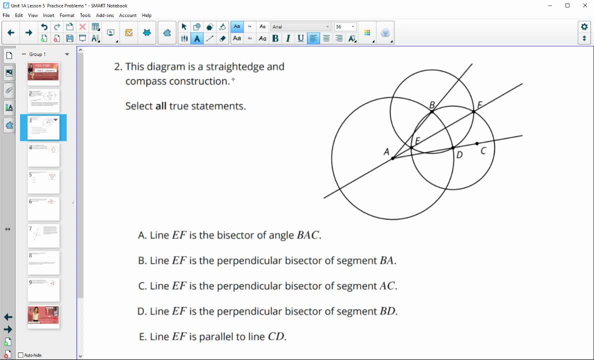 Number two in this diagram is the straight edge and compass constructions. Select all true statements. So this one is the construction of the angle bisector, if you remember. So let's take a look here. So it says line EF. So here is line EF. 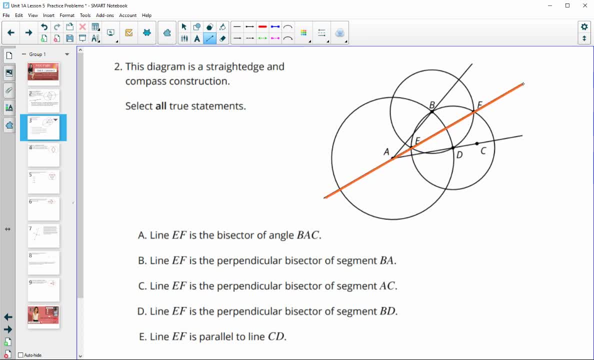 It's this line. So is line EF the angle bisector of BAC? Yes, it is. If you remember, we just constructed that in lesson five. Line EF is the, so the same line. is this line the perpendicular bisector of? so is it the perpendicular bisector of this segment? 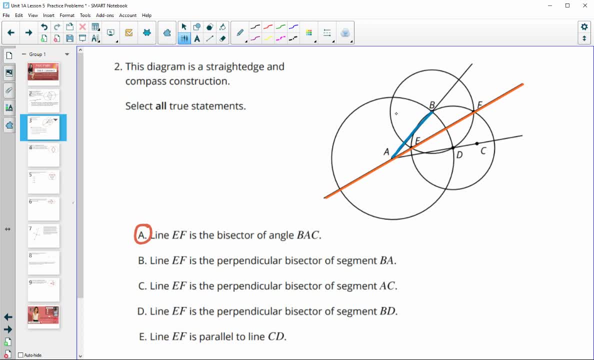 So it would have to hit this segment at a 90 degree angle through the midpoint. So that would be like right there. So this is definitely not the perpendicular bisector of AB. Is that line, EF, the perpendicular bisector of AC? Again, no. 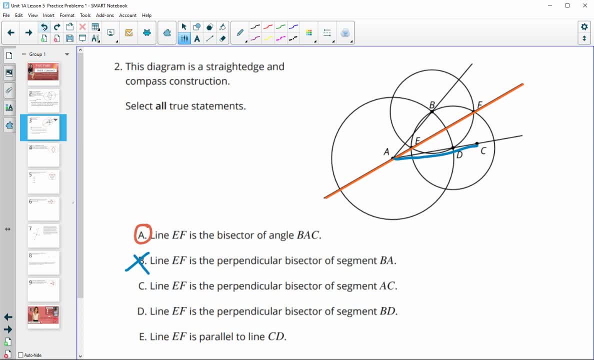 The midpoint would be somewhere about here and go this way. So that is not true. Is EF the perpendicular bisector of BD? That is true. And then is EF again this orange line? is it parallel to AC? Remember, parallel means two lines that never intersect. 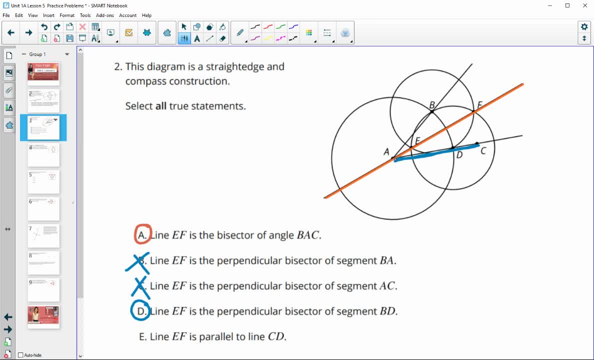 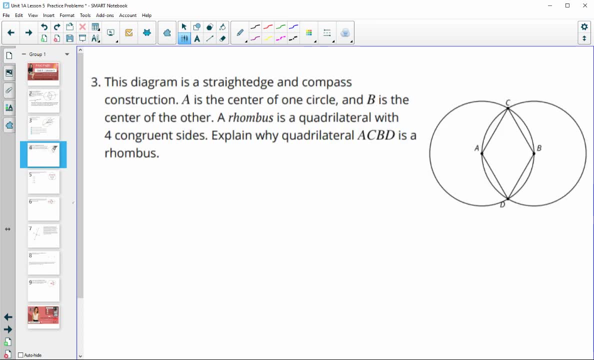 So since CD does intersect EF here at A, these would not be parallel lines. Number three: This diagram is a straight edge equation. This diagram is a straight edge and compass construction. Again, A is the center of one circle, B is the center of the other. 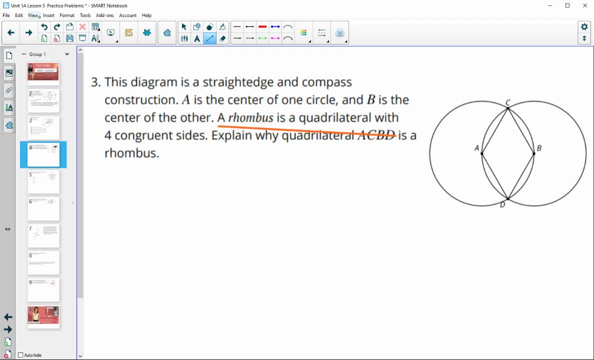 A rhombus is a quadrilateral with four congruent sides, So explain why ACBD. so this quadrilateral here is a rhombus. So how do we know, essentially, that all of those sides are congruent? How do we know that all of those sides are the same length? 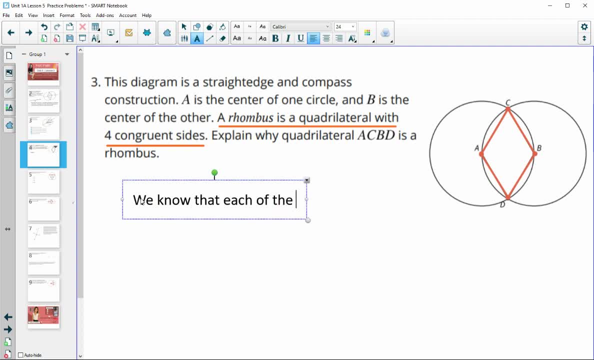 So we know that each of the sides of ACBD are radii of congruent circles. So they are congruent. And you might want to add in how you know that the circles are congruent. So I'm just stating that they're congruent, right here. 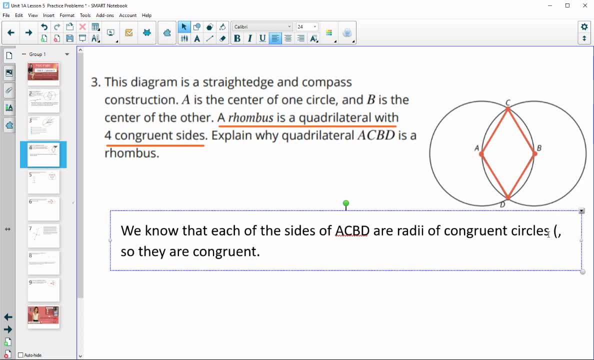 But you could also add in, how you know, both circles are congruent because they both have AB as a radius. So both circles have a radius length of AB, which means that they have to be the same because their radii are the same Number four, AB and C are centers of the three circles. 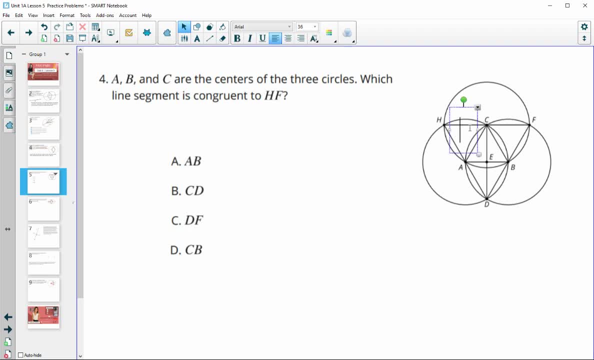 Which line segment is congruent to HF? So which one here is congruent to HF? So is it? let me see what I have here. So is it AB? And that's not true. So AB is just a radius, HF is a diameter. 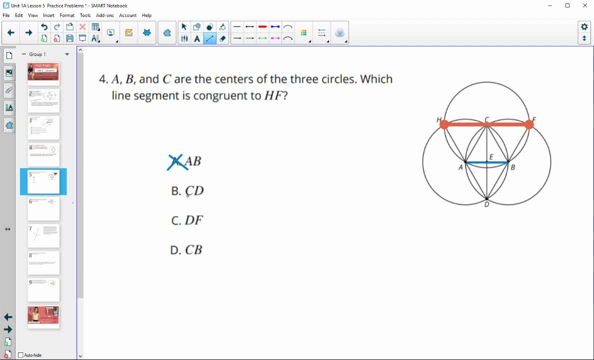 It goes all the way across the circle, through one of the centers. Is it CD? So CD is just a chord. It doesn't actually go through the center of a circle. So it's not a diameter, So it's not CD. DF. 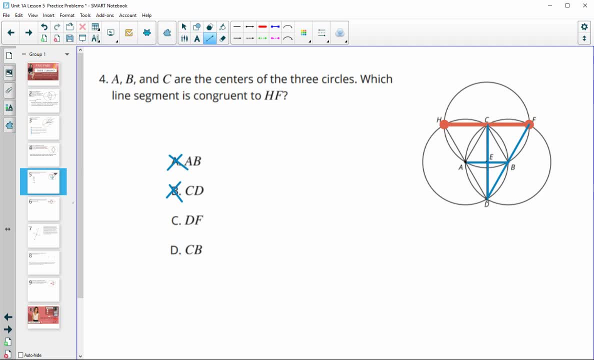 So DF does go from the edge of a circle to the other edge And it goes through point B. So DF is a diameter as well. So DF and HF are congruent to each other, And then we can just check CB. Let's see. 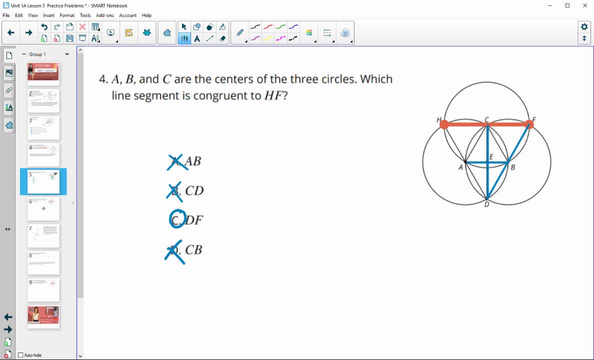 It would be a radius not congruent. Number five in the construction: A is the center of one circle, B is the center of the other, So essentially those two circles are equal. Explain why segment EA is the same length as BC. 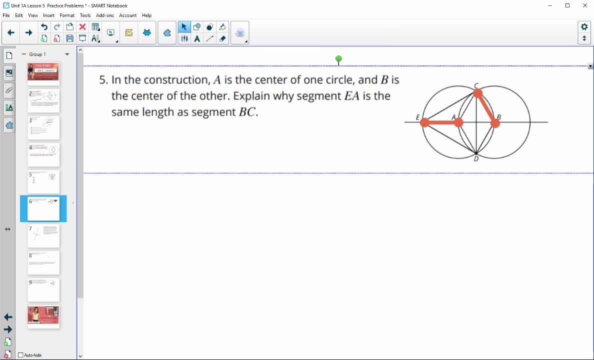 So if we look there, we see that they are both radii, So both are radii of congruent circles. So if we look, this goes from A to the edge, so center to edge. This one goes from center to edge as well, B to C. 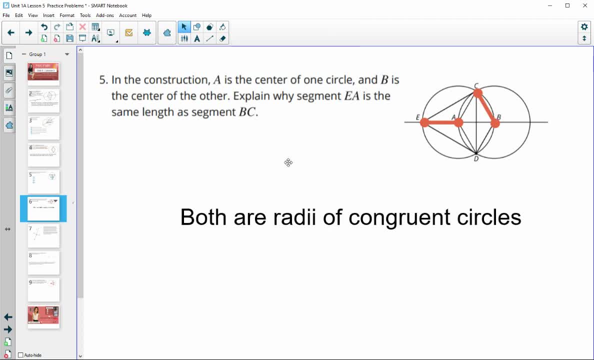 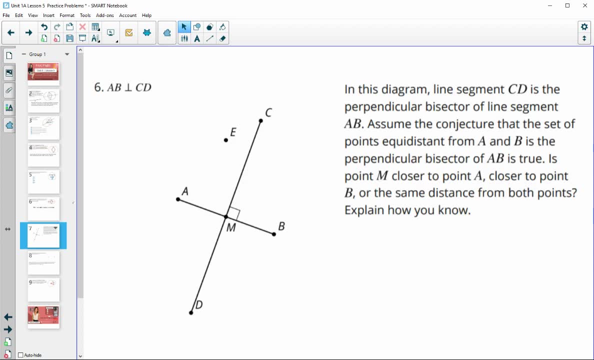 And the circles are the same size, So radii in congruent circles are going to be congruent to each other. Number six: in this diagram the line segment CD is the perpendicular bisector of AB, So CD is bisecting AB. 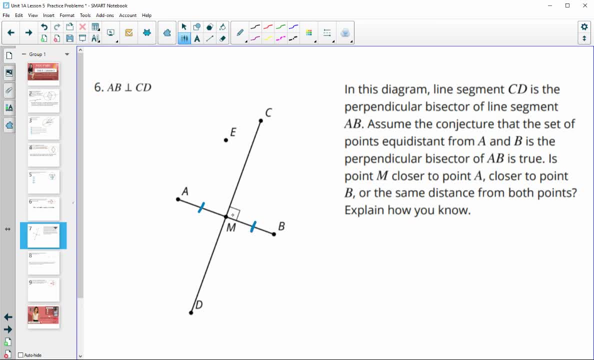 So I like to split that, put the little tick marks and then you see the 90-degree angle. So assume the conjecture that the set of points equidistant from A and B is the perpendicular bisector. So everything. let me draw this line on here. 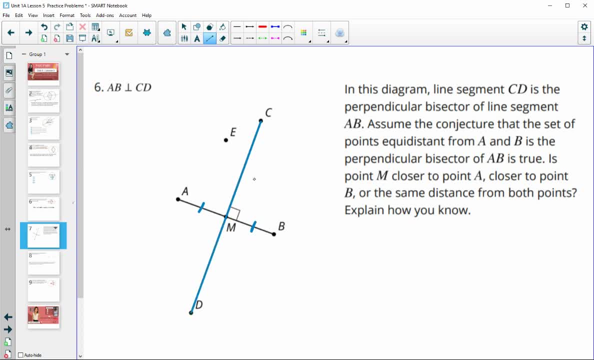 So everything on this blue line is the same distance from A. Any point on this line is the same distance from A as it is from B. So is point M equal? Is point M closer to A, Is M closer to B, Or is it the same distance from each one? 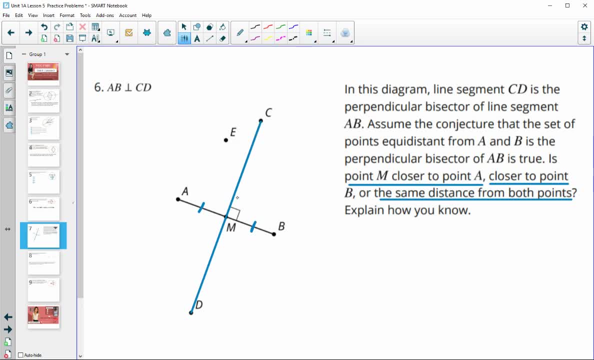 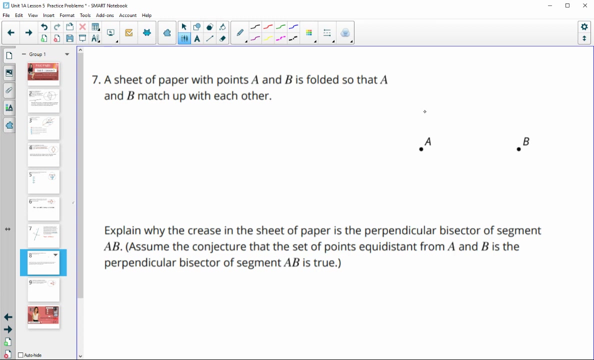 So here is point M. So is M closer to A, closer to B, or the same distance? So M is the midpoint, so it's the same distance. All right, number seven: a sheet of paper with points A and B is folded so that A lands on B. 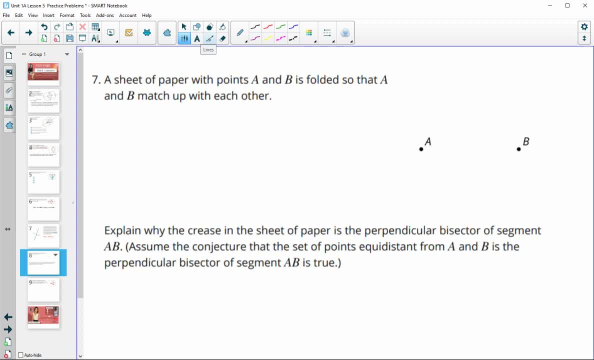 Explain why the crease on the sheet of paper. so let me just kind of draw this crease. Okay, so we're going to get this crease on the sheet of paper. Explain why the crease on the sheet of paper is the perpendicular bisector. 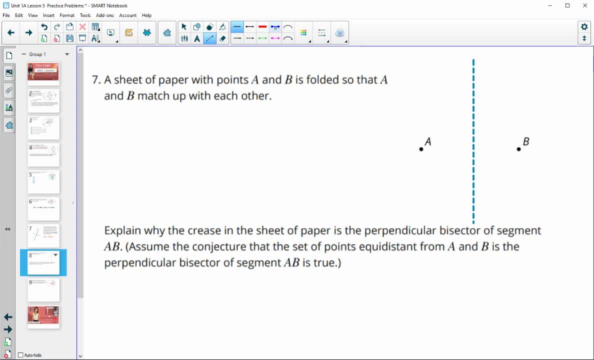 So if we think about this, I'm just going to draw this, I'm just going to draw this out a little bit more here. So I'm going to draw the other edges of the paper as we fold it. So I'm going to fold A over onto B. 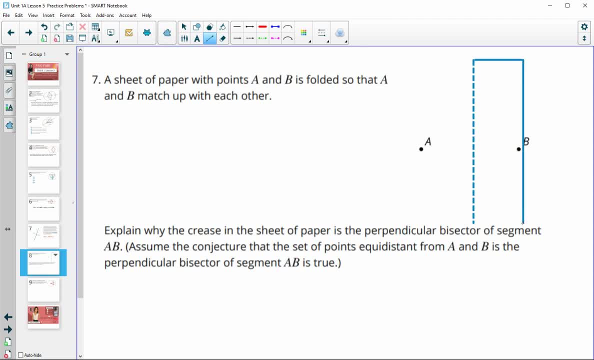 So if you can imagine this paper just folding over- I'm going to move it a little so it goes through- All right. so if we had folded this piece of paper over, so that point A landed right on B, so now, if you imagine, this flipped right over. 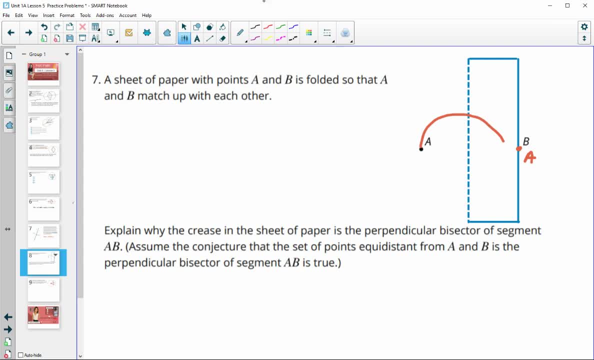 so now A is landed on B And then here's the paper. And why don't I even get rid of A here? so we can't even see it. So we're going to fold it over. so it folded over right there on top of B. 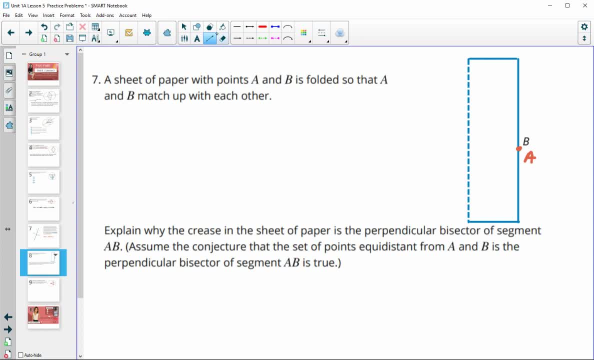 So now, as it's folded over, we could just draw a point here, okay, a point anywhere on this fold, And I'll just call it C, And we could connect that point to A and B at the same time, So it's simultaneously on both of these points, because this is still folded.